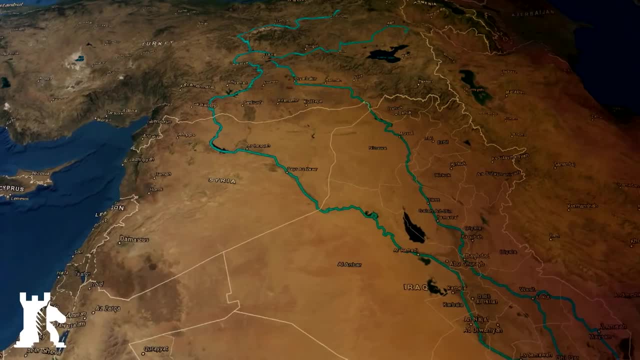 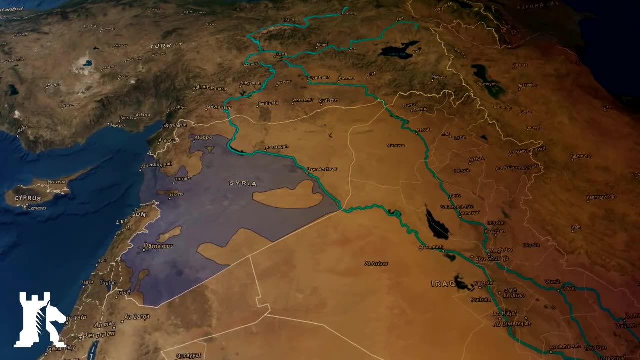 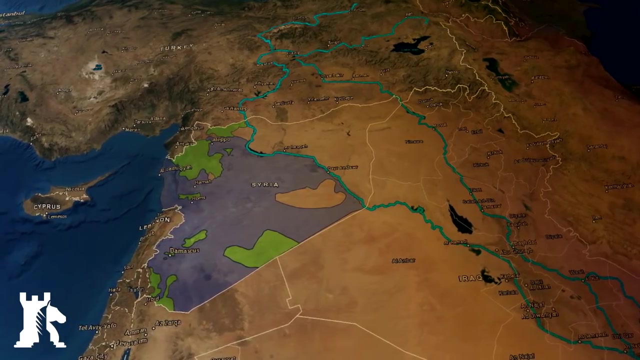 but the involved nations are divided into a number of camps. On one side is a coalition of Iran, Russia and the Al-Assad government. On the other is Turkey and the Syrian National Army, which is a coalition of former Free Syrian Army militias and Islamist groups. 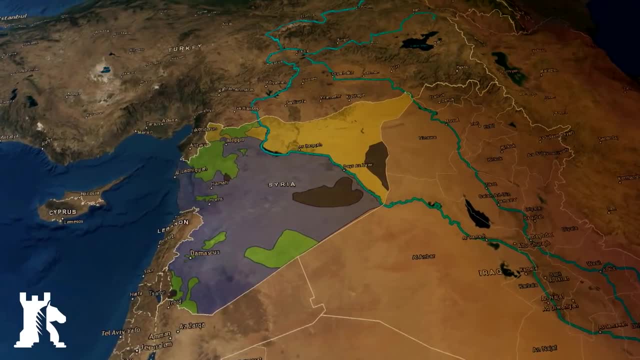 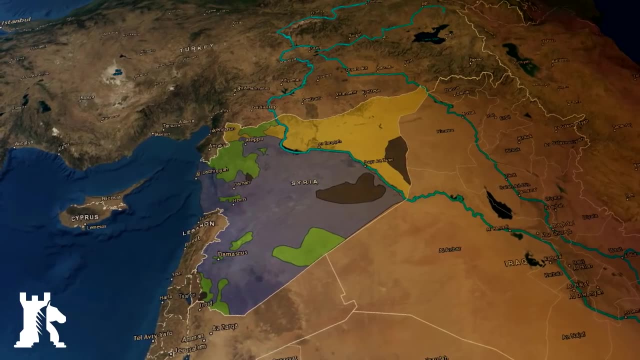 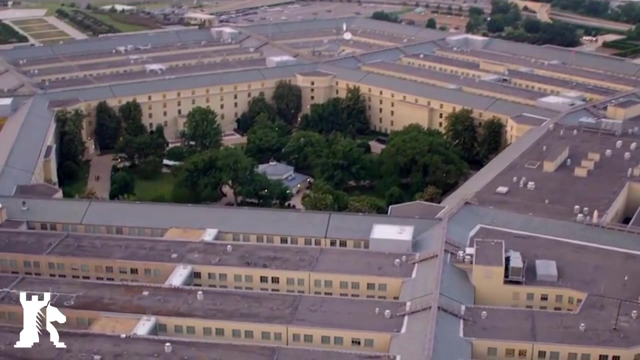 Meanwhile, Washington uses the Kurdish militias to bolster its separate voice in the conflict. Considering these lines of division, it's safe to say that the only relation the conflict has to Syria is that it happens to be taking place there. This notion was further reinforced by the Pentagon on January 13th. 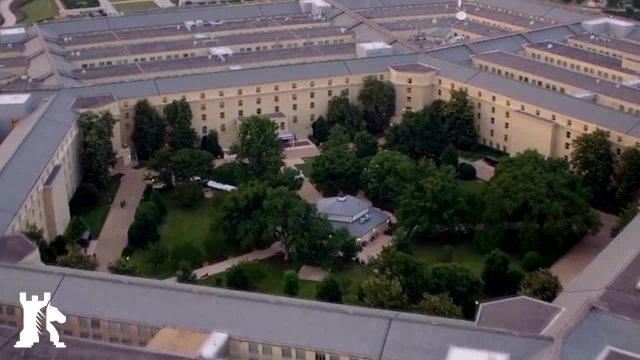 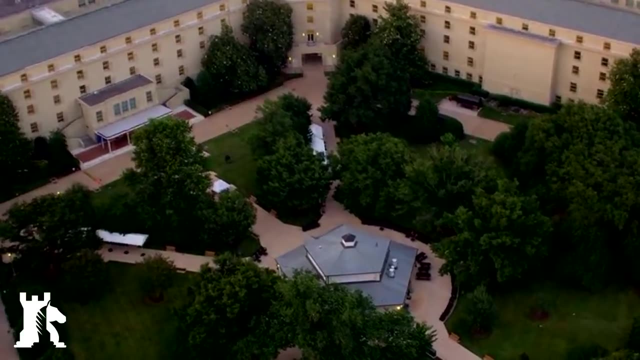 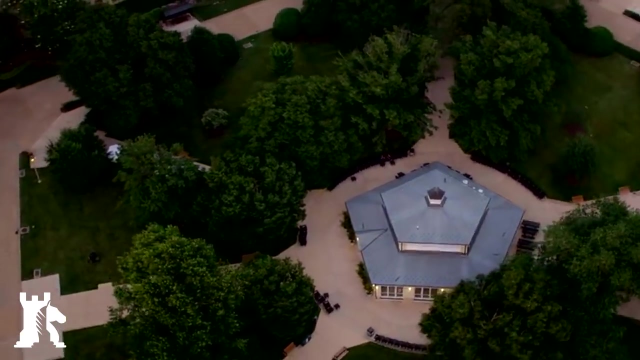 when it was revealed that the CIA seeks to create a new 30,000 strong border security force in the Kurdish-controlled territories in Syria. The official mission is to prevent ISIS from regaining a physical presence in the region, but in truth, Washington hopes to retain a significant voice in the conflict. 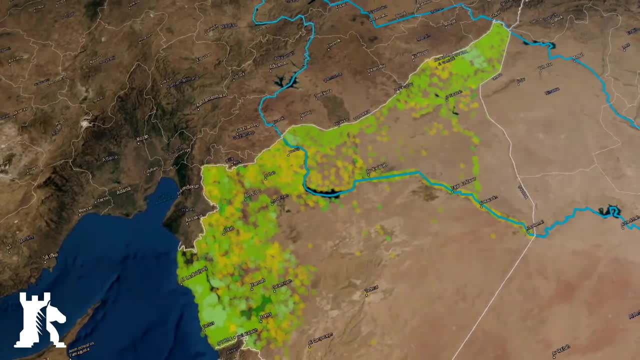 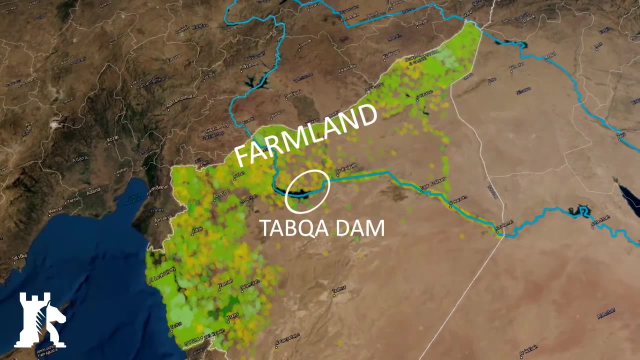 The fact of the matter is that the Kurdish militias occupy Syria's finest agricultural land, and the Kurdish-controlled Tabqa Dam on the Euphrates provides half of the country's energy output. Since the Syrian-based Kurdish militias are the only ones in the conflict, 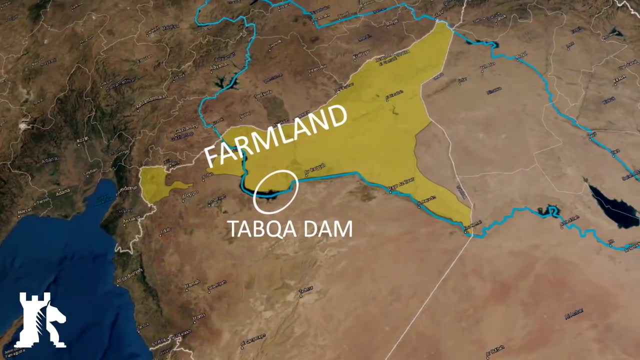 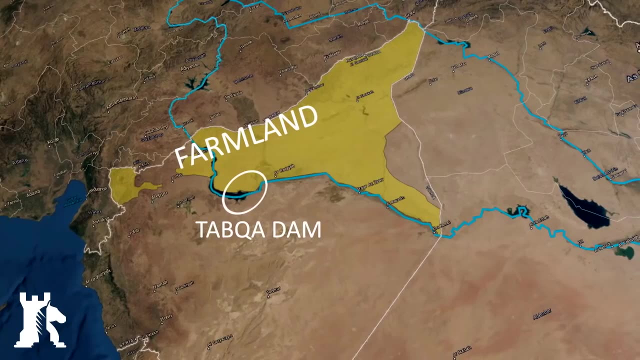 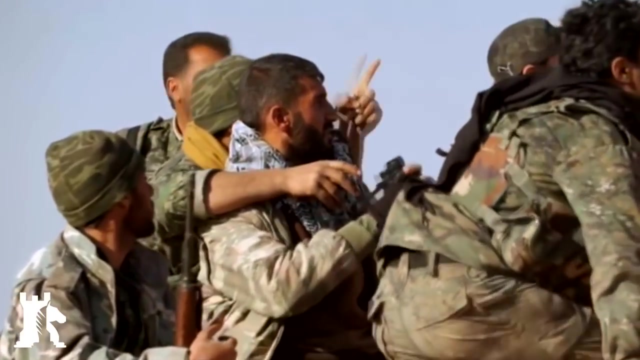 it means that Washington can dispossess Syria of capital and energy resources. In this context, the plan to strengthen the Kurdish militias ultimately serves the Americans. What's more is that the United States embedded about 2,000 American military personnel in the Kurdish YPG units near Manbij and the Kurdish-controlled territories east of the Euphrates River. 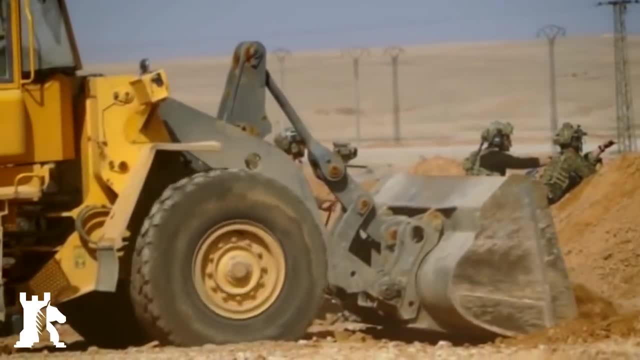 The purpose behind this is to create a new, more efficient and more efficient Kurdish territory. The Kurdish YPG units are the only ones in the conflict and the Kurdish YPG units are the only ones in the conflict. The Kurdish YPG units are the only ones in the conflict. 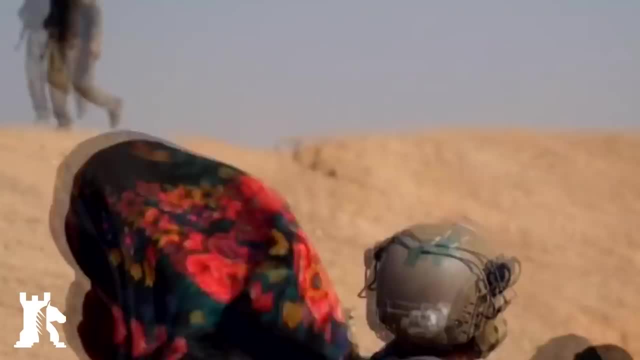 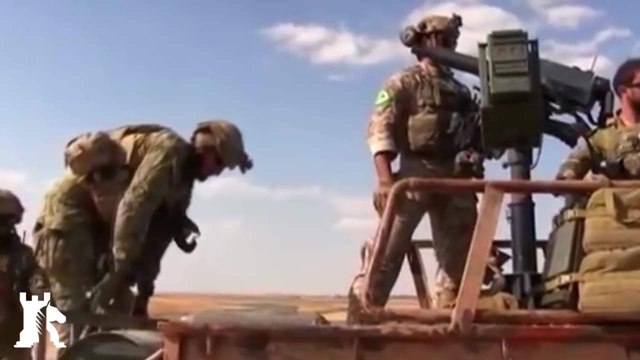 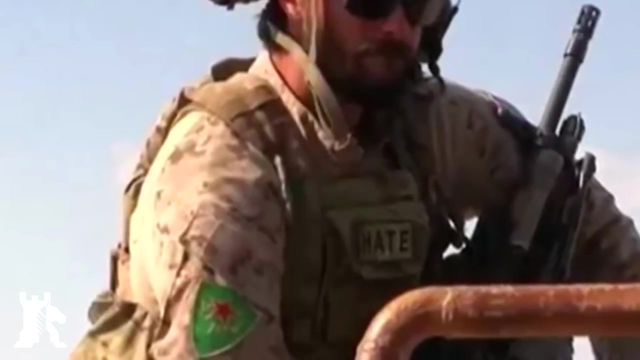 The purpose behind this was to deter a Turkish, Russian or Iranian attack on the Syrian Kurds, and it worked. None of the other powers wanted to accidentally attack American military personnel, which would have given Washington political leverage. By this practice, Washington essentially uses its embedded military personnel. 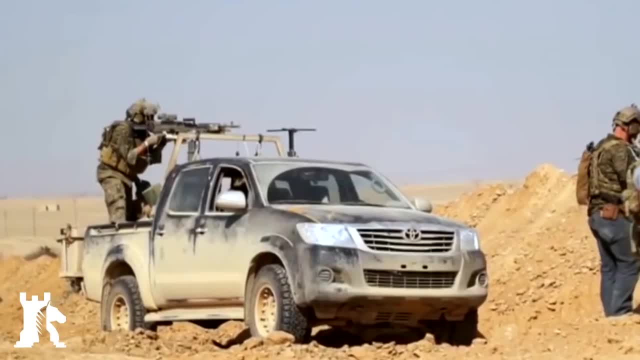 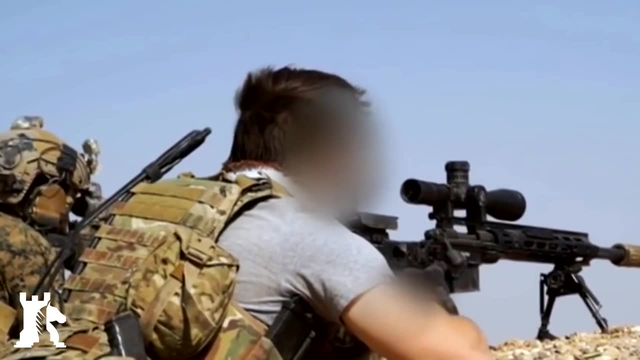 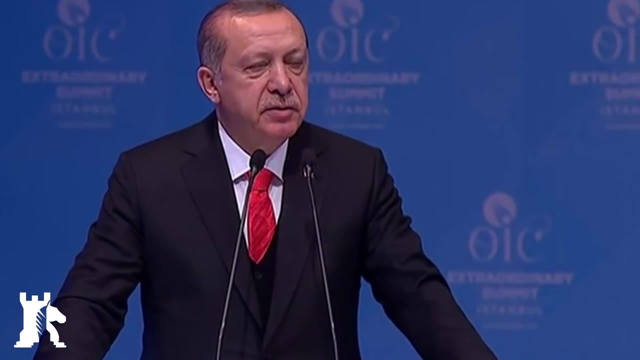 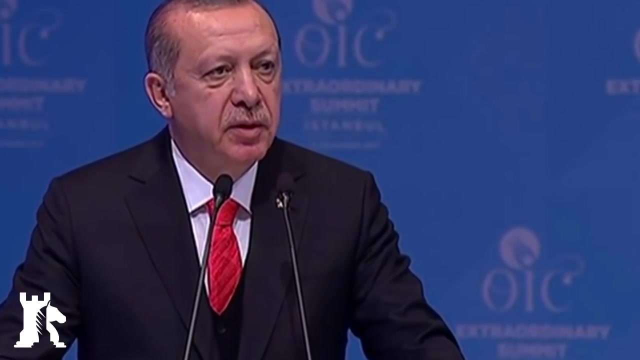 as provocative pawns in a game of chess. However, such tactics and the policy concerning the new Kurdish army has driven a wedge between Ankara and Washington. Immediately following the Pentagon's announcement, Turkish President Erdogan pledged to strangle such designs. For Turkey, the primary focus is to contain the influence of the Kurdish militias. 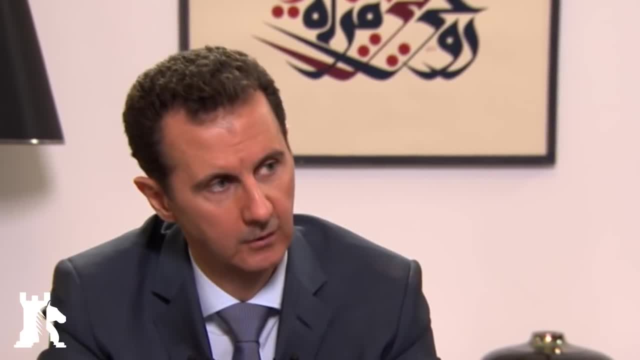 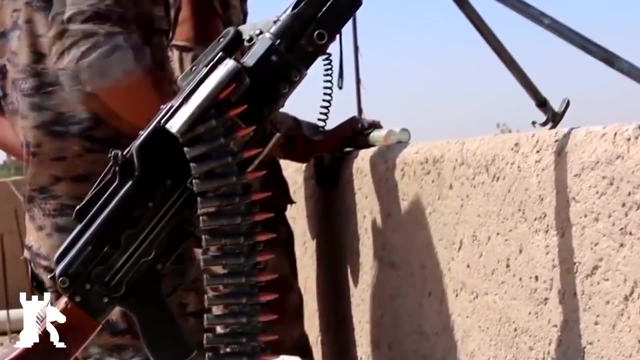 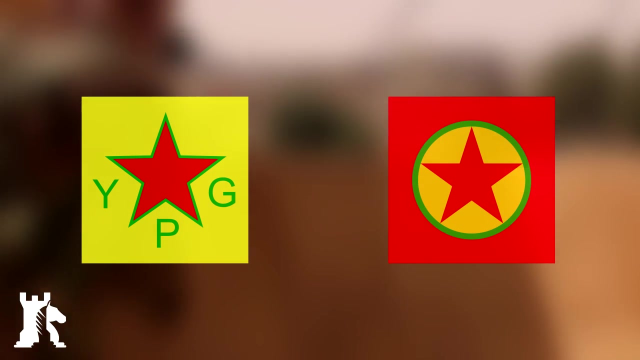 as opposed to regime change in Damascus. In this framework, the American program is a threat to Turkey's sovereignty, since the ranks of the new border security force would exist mostly of YPG units, which has indisputable ties to the PKK, which is a widely designated terrorist group that has carried out attacks. 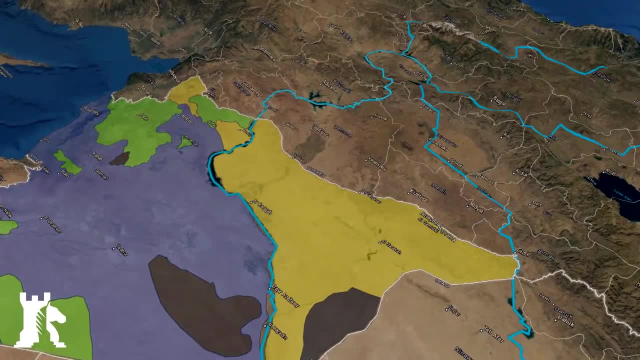 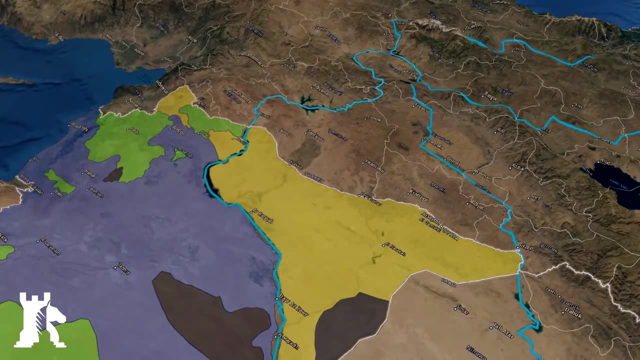 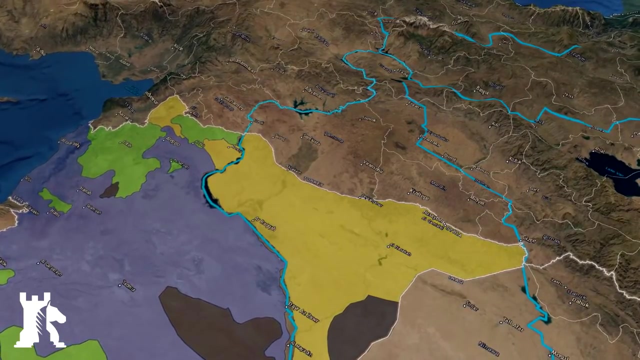 in Turkey over the past few decades. So Turkish policy makers fear that a strengthened YPG presence in Syria could harbour PKK members who seek to launch attacks into Turkey. These concerns are valid in their own right, For instance, the YPG-controlled Afrin enclave in. 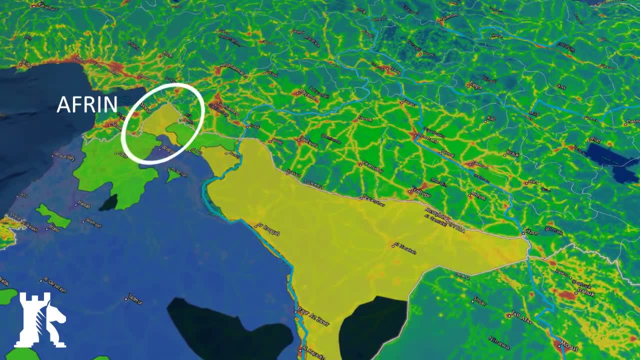 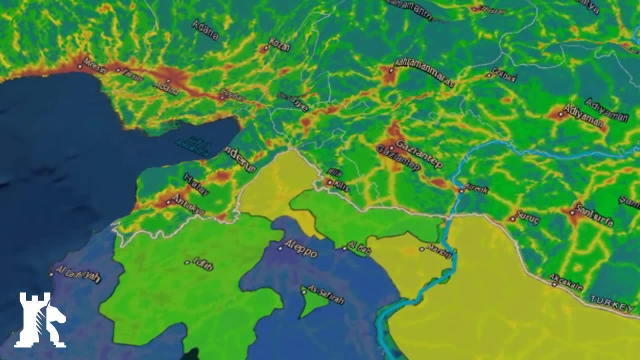 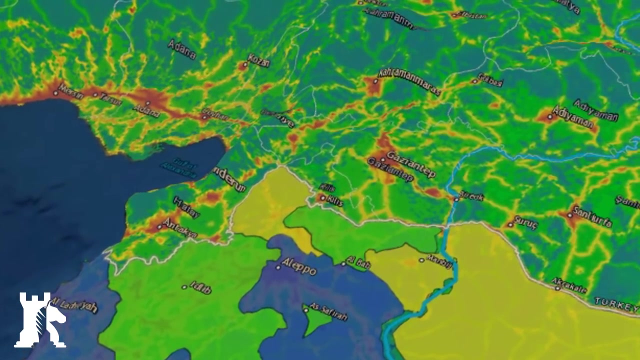 northwest Syria is in close proximity to Turkey's densely populated regions of Gaziantep and Hatay. So, considering the facts on the ground, the government in Ankara does not want the PKK and YPG to gain more ground, which is why the Turks recently launched an assault on Afrin. 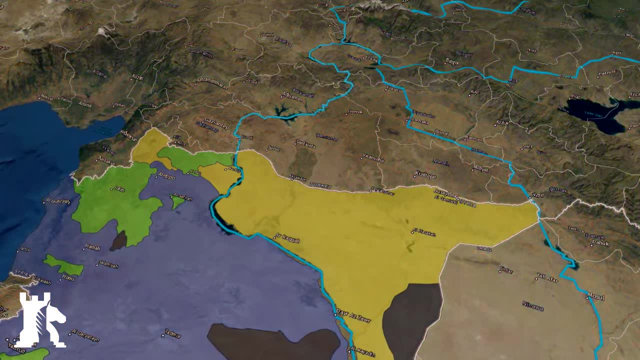 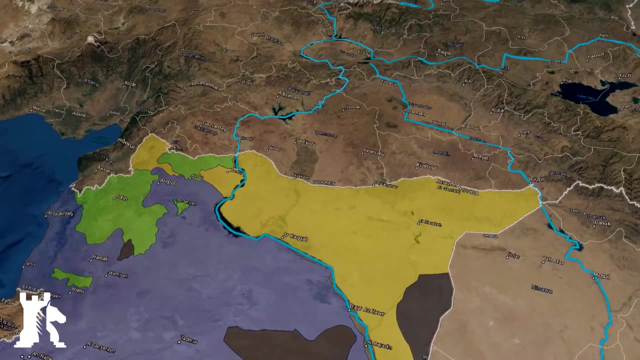 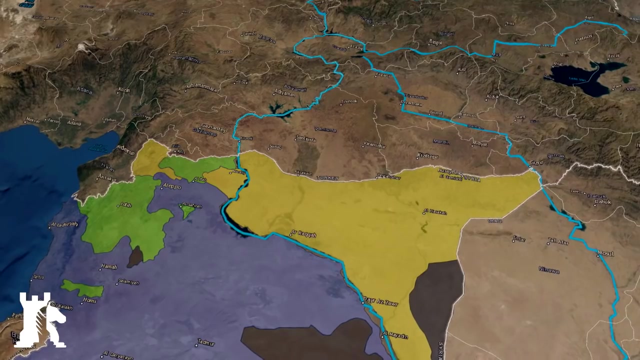 This unusual turn of events displays just how much the status quo has changed over the years. Even supposedly allies and partners such as the Kurdish-controlled Afrin enclave have been able to get in touch with the Kurdish-controlled Afrin enclave. The situation in Afrin is further complicated by the involvement of Moscow. 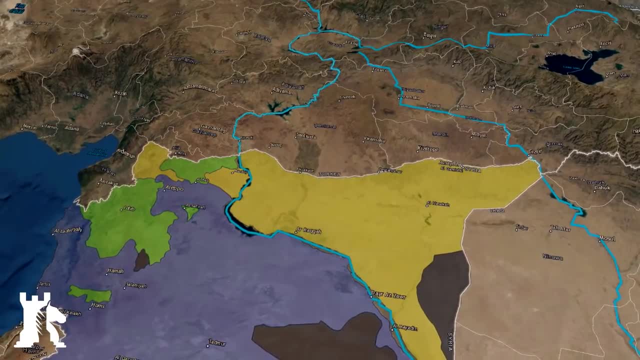 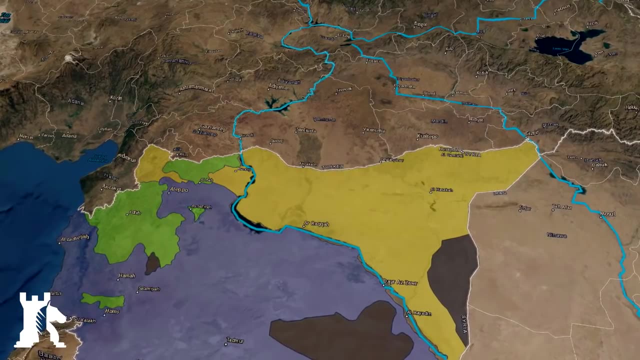 Just as Washington has placed American military personnel in the YPG contingents east of the Euphrates, Russia has embedded its troops in the YPG units in the Afrin enclave. So, while the Kurdish-controlled regions east of the Euphrates river, 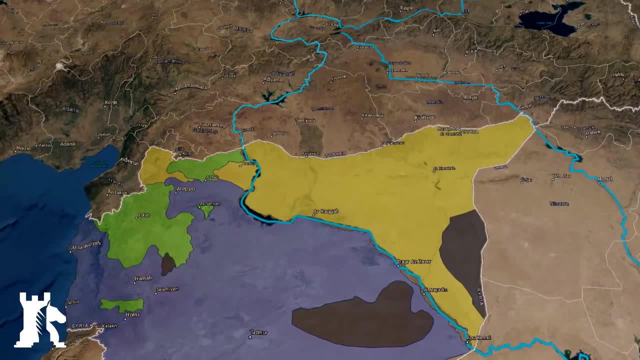 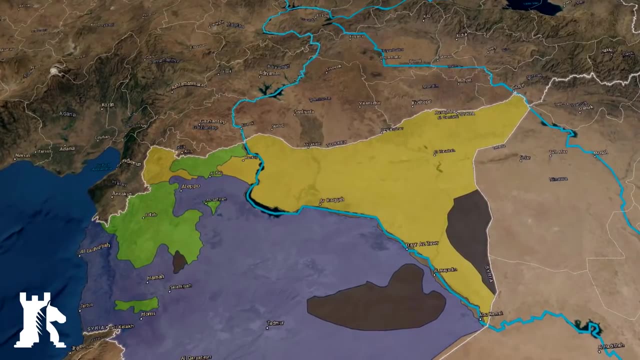 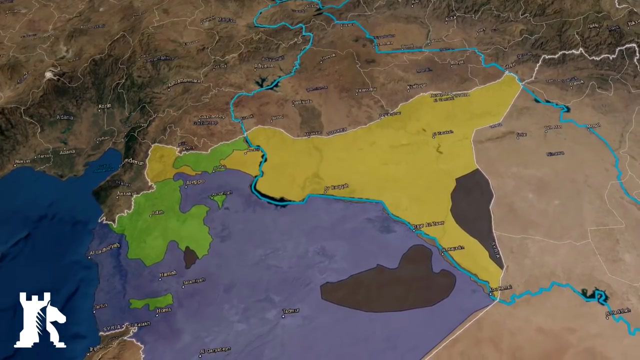 are part of the American sphere of influence. Russia is part of the Russian sphere. What has changed as of January 2018 is that the Russian military forces have either left Afrin or conceded the enclave to Turkey. Either way, the exit of the Russians has decreased the chances of an accidental skirmish. 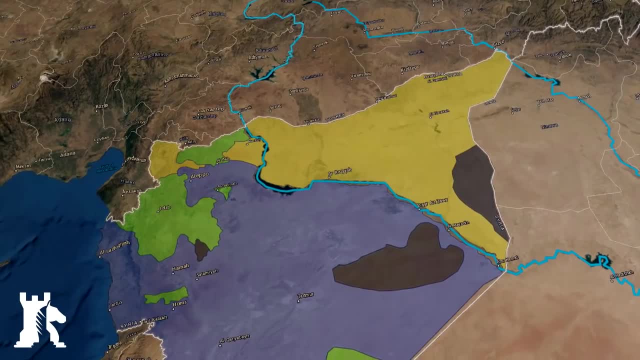 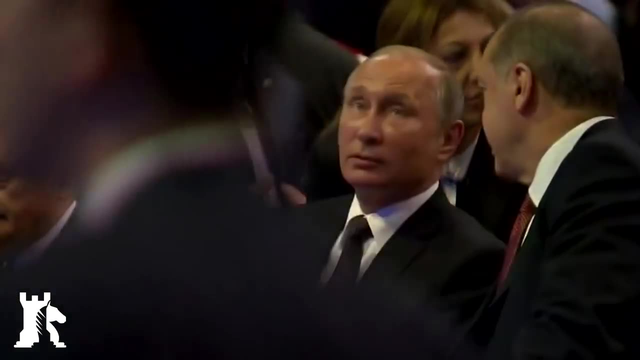 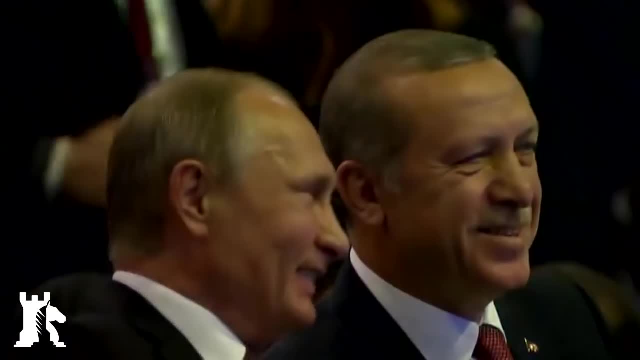 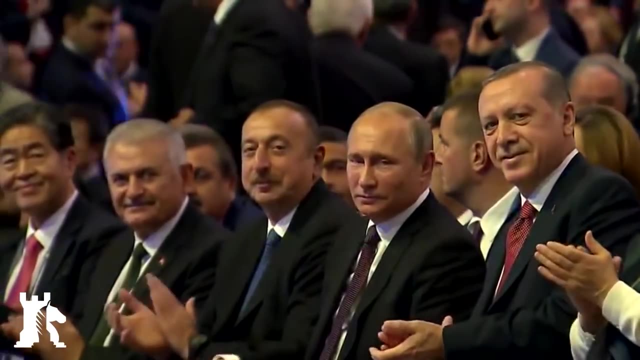 What exactly incited Moscow to attack the YPG in Afrin? What exactly incited Moscow to attack the YPG in Afrin? But what is certain is that, for the past year, Erdogan and Putin have conducted several talks concerning a political resolution to the conflict in Syria. 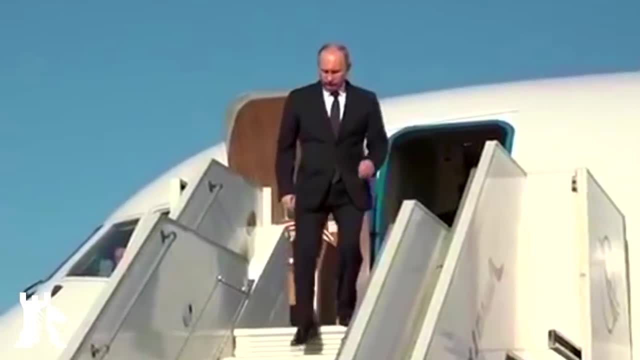 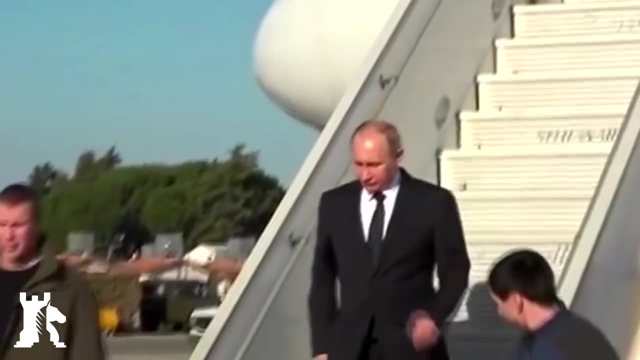 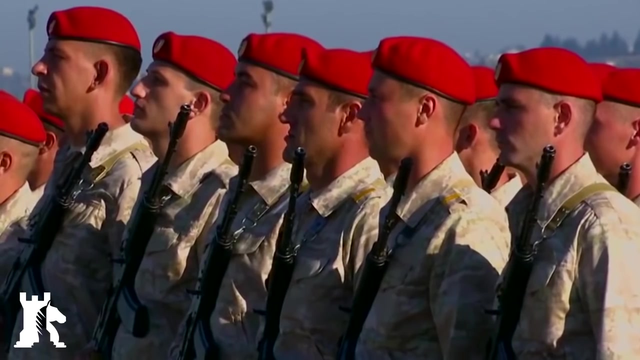 As fighting has continued, an increasing number of Russian analysts believe that a military victory in Syria will require years of additional intervention. This is something that Putin cannot afford, nor does he want to. The Russians do not want to make the same mistake as the Americans did in Iraq and Afghanistan by aimless occupation. 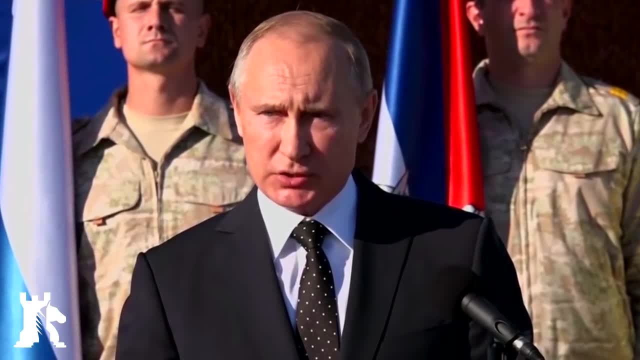 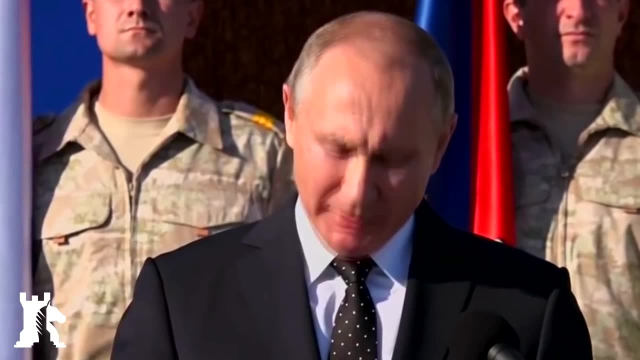 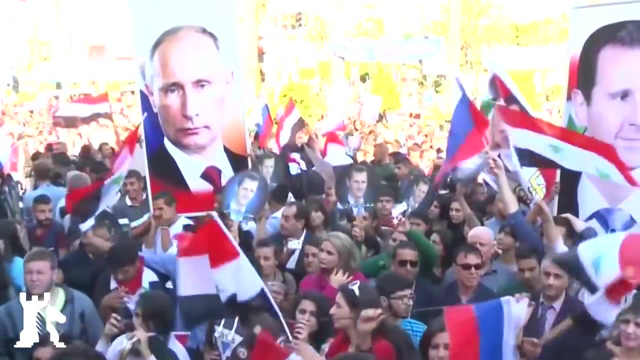 So, for the past two years, Russia has been searching for an exit without losing its gains on the ground. It tried to reach an understanding with the United States, but those endeavours failed. So instead, starting from September 2017,, Russia has sought to disengage itself from Syria. 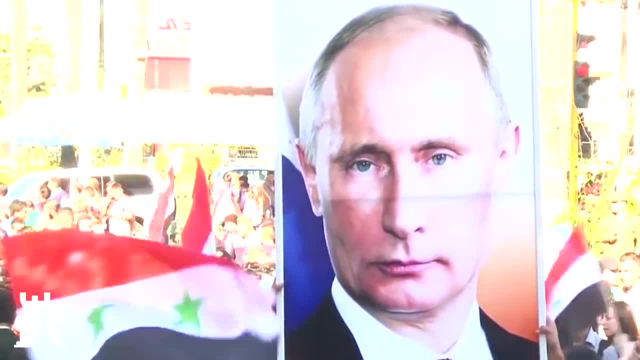 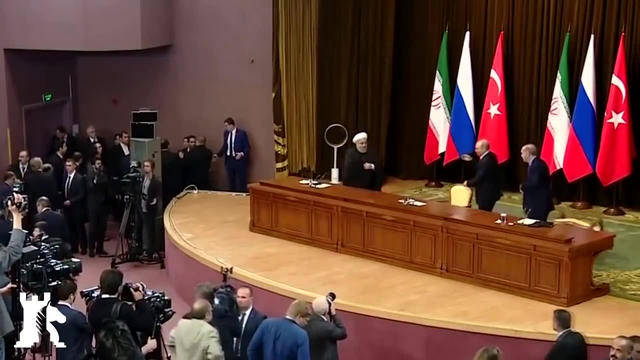 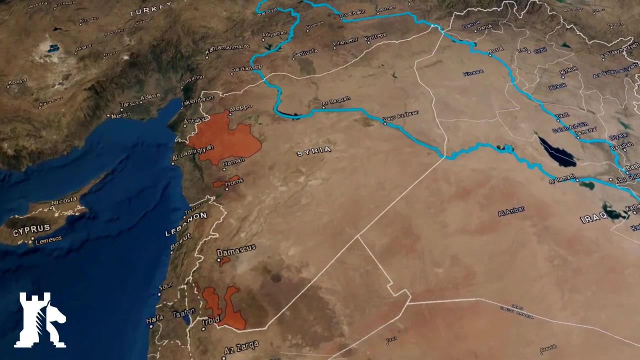 by negotiating a political resolution to the conflict. These negotiations laid the bedrock for the Astana peace talks, where Turkey, Russia and Iran reached an understanding last year in the capital of Kazakhstan. The parameters of the Astana agreement prescribed the setup of four de-escalation zones in Syria. 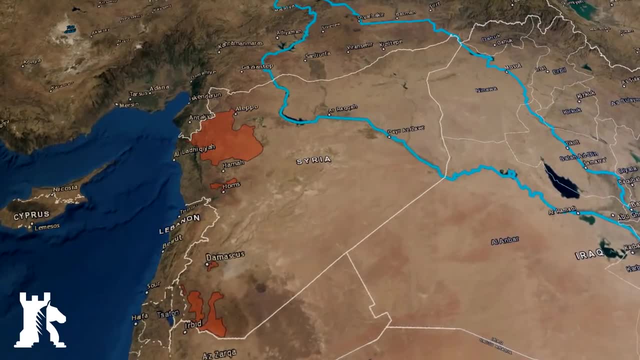 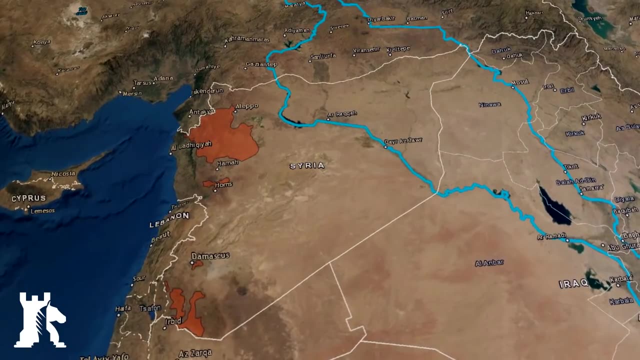 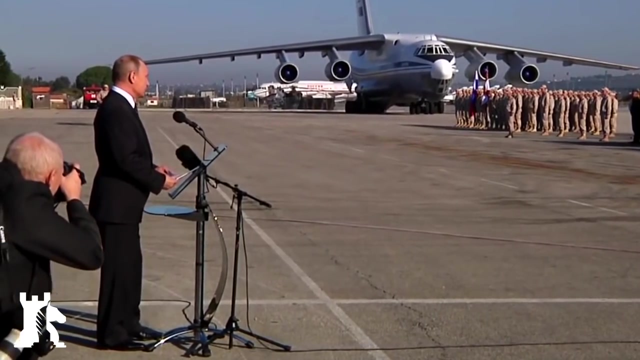 that would cease hostilities for a period of six months. For a moment, a political solution seemed within reach, and the Astana talks shifted the Syrian crisis from military to diplomatic, to diplomatic ground. In anticipation of this, Putin visited the Russian airbase in Syria. 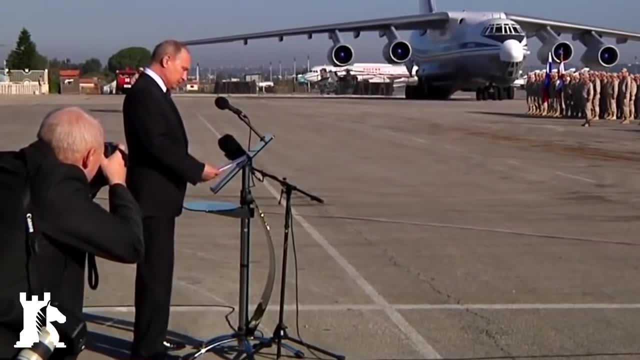 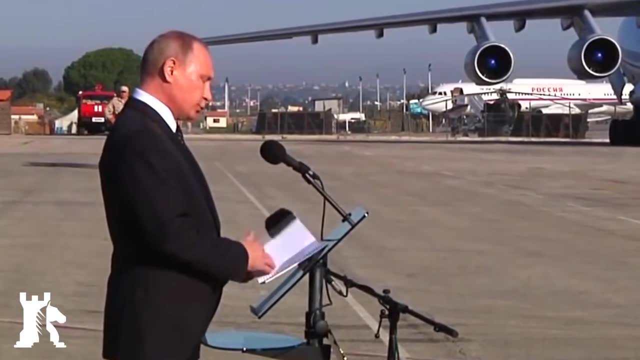 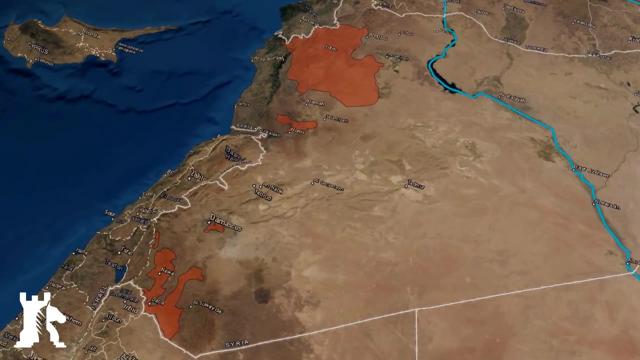 where he proclaimed the imminent retreat of Russian forces. However, as is the case with all coalitions, the more members there are involved, the more tedious the political proceedings become. First, there was disagreement over Turkey's right to station its forces in the Idlib region. 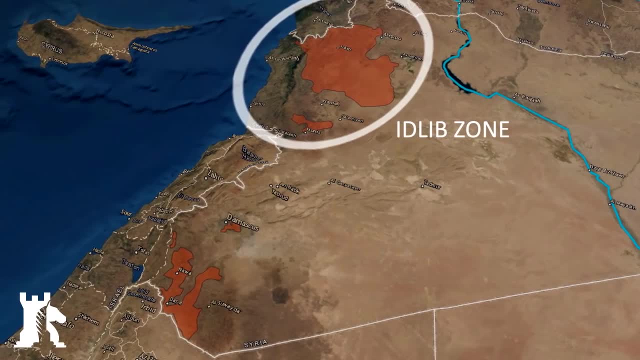 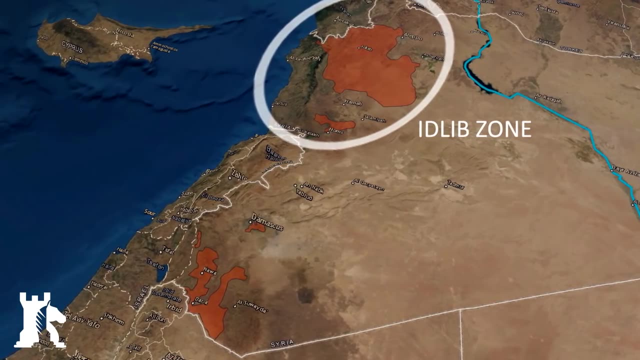 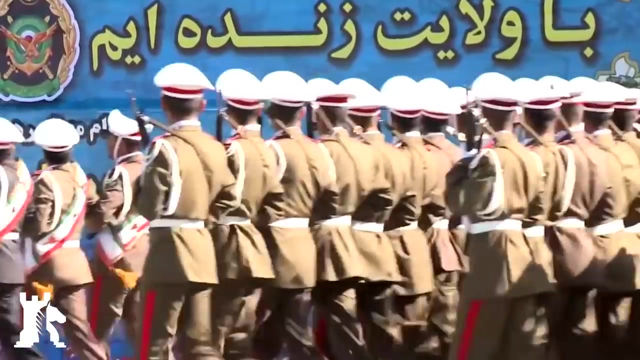 and whether the Turkish-backed Islamist militias counted as terrorist groups and must then provide России with necessary resources in order to stop Turkey and Russia from use a military force that would continue to be targeted by the other powers. Second, the government in Tehran disagreed over the size of the Idlib de-escalation zone. 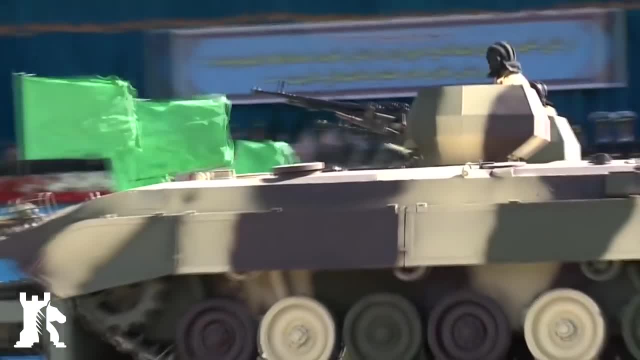 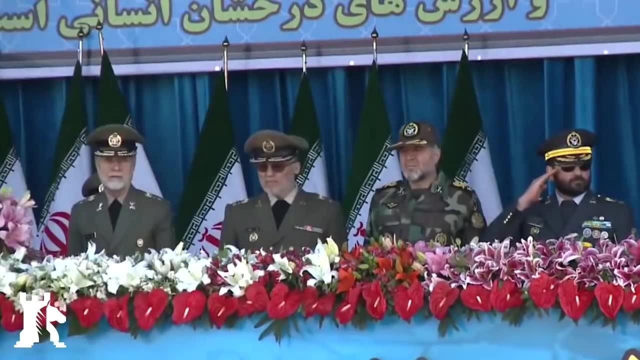 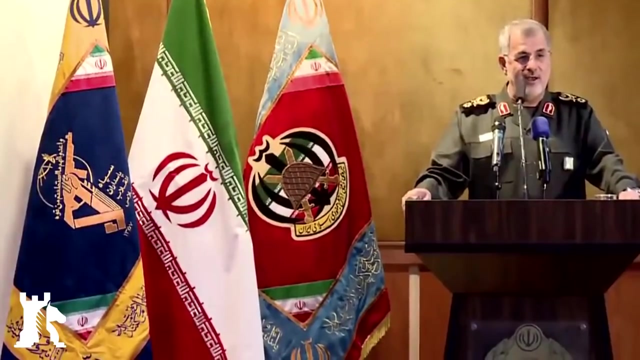 More to the point, Iran was not really interested in a negotiated stalemate, because it sees Syria as an essential part of its geopolitical policy. The Iranian's have also committed far more resources to the Syrian war effort, shown support in the form of air power and diplomacy. Iran, by comparison, has mobilized 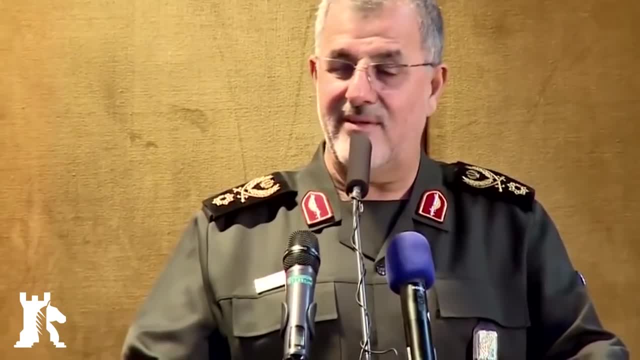 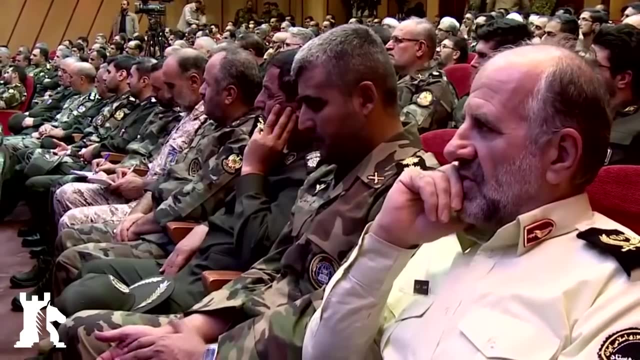 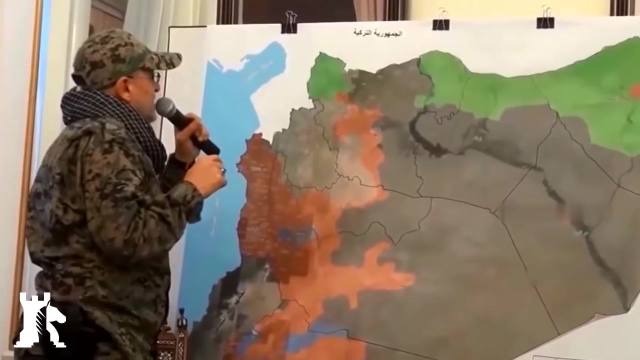 thousands of its proxy militia fighters to enhance the ranks of al-Assad's forces. Tehran has also helped to keep the Syrian economy afloat by financial means. So, unlike the Russians, Iranian policymakers are committed to a complete military victory in Syria, regardless of the costs. This 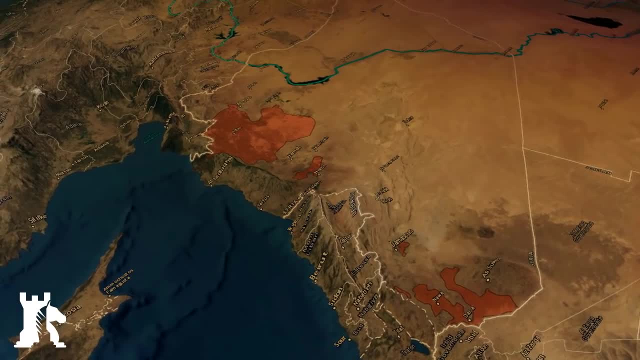 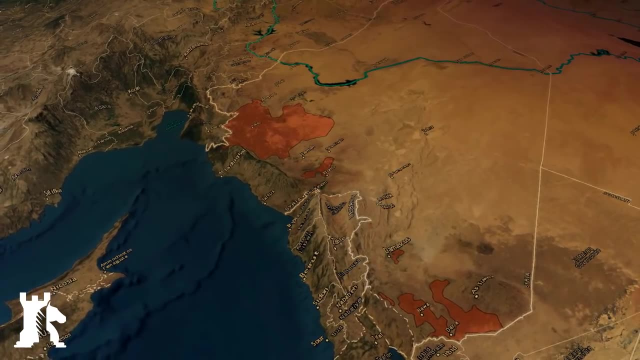 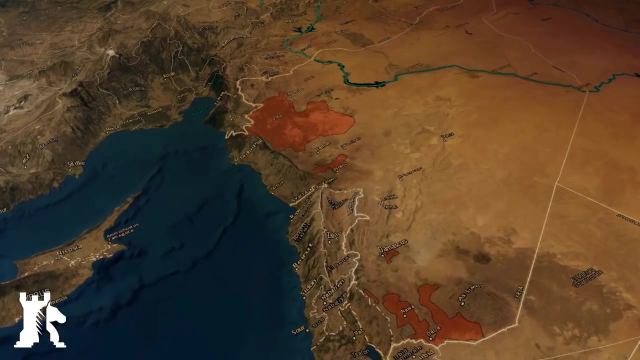 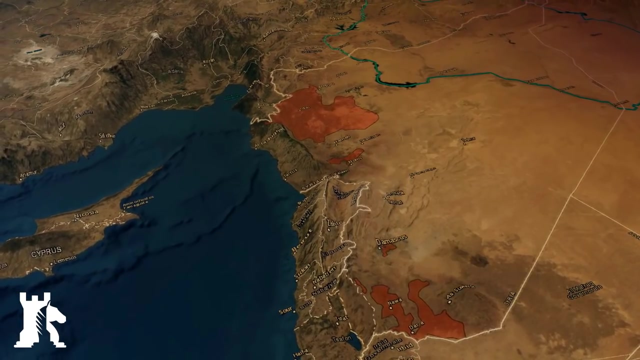 divergence in interests is similar to the Turkish-American policies on Syria and, just as Washington and Ankara undermine one another, Tehran also undermined Moscow's peace efforts. More specifically, in early January, while the Russians and Turks were negotiating the finer details of the Astana ceasefire, Iranian-backed proxies and al-Assad's elite forces derailed the 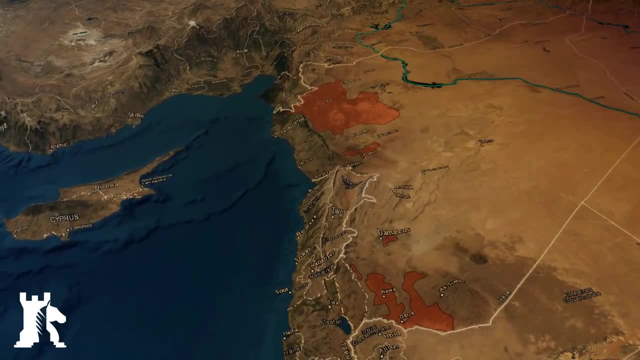 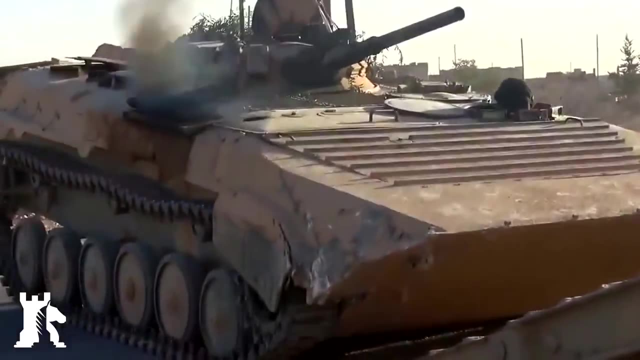 peace talks by striking the agreed-upon de-escalation plan. At the same time, some Turkish-backed rebel forces also breached the Astana ceasefire, For instance Hayat Tahrir al-Sham, which is the most dominant militant group in Idlib, whose 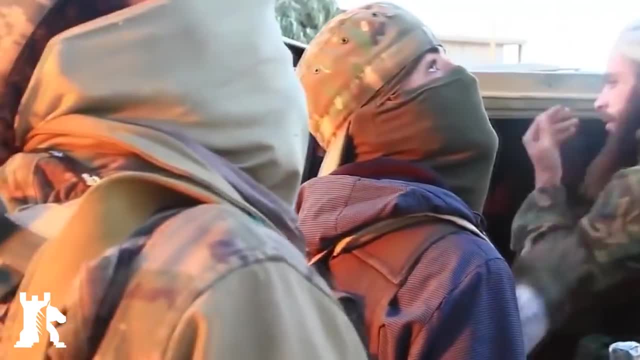 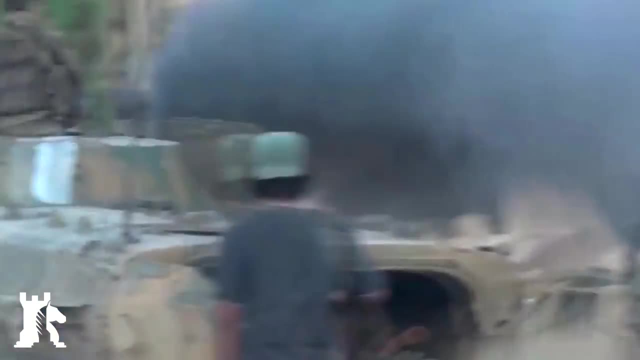 core elements are part of. Al-Qaeda, refused to abide by the ceasefire and launched offensive operations on al-Assad's forces near the city of Hama. In the same period, a swarm of unidentified satellite-guided drones attacked the Russian air force. The Al-Assad's forces were also. deployed in Syria, which was another breach of the ceasefire. Initially, blame was cast on Turkey, but Putin later clarified that the Turks were not the perpetrators. To this day, it's still unclear who was behind the drone attack. For all its shortcomings, the Astana ceasefire was the biggest. diplomatic breakthrough in the Syrian war in years, But the recent Iranian breach of the ceasefire, the drone attack on the Russian airbase, the American setup of a new army and the Turkish military operation in Afrin has reignited the conflict and brings out the contradicting policies out in the open.